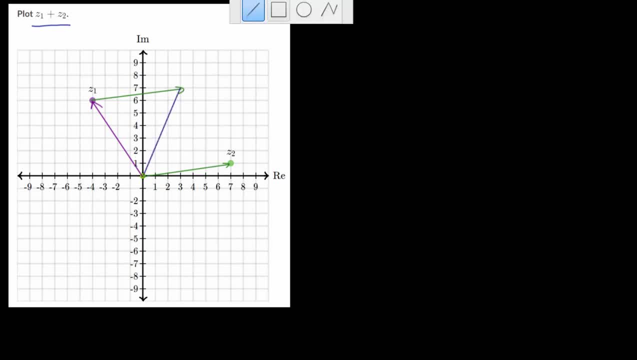 and that will start at the origin and go all the way up to this point here. so this blue vector, this is just Z 1 plus C 2 and we can figure out where that ends. it looks to be at the coordinate three plus seven. I where three. 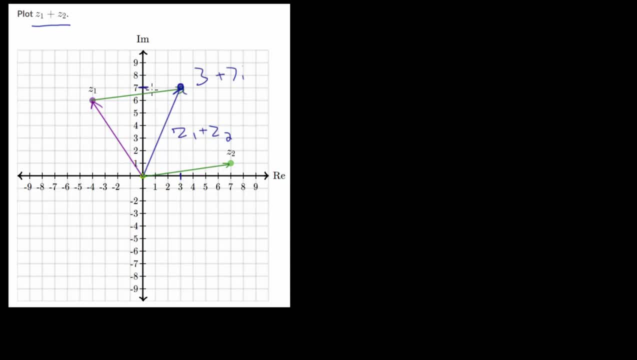 that's the real part, and seven I. that's the imaginary part. so it looks to be that this is the answer and, of course, the way to check this is to rewrite both your vectors in terms of their real and imaginary parts. This is, excuse me, 7. 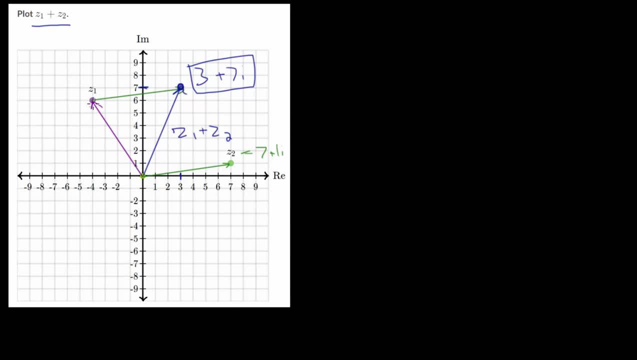 plus 1i and this vector z1, this is minus 4 plus 6i. And when writing it like this, we can just now add, using arithmetic: We add the real parts minus 4 plus 7,, that's 3, and we add the imaginary parts. 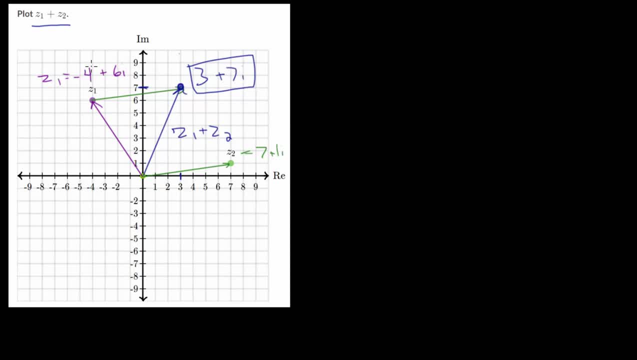 6i plus 1i would give us 7i. So either way you want to approach this, we'll get this exact same answer: 3 plus 7i, and using both methods is a great way to check this. Now let's do one final. 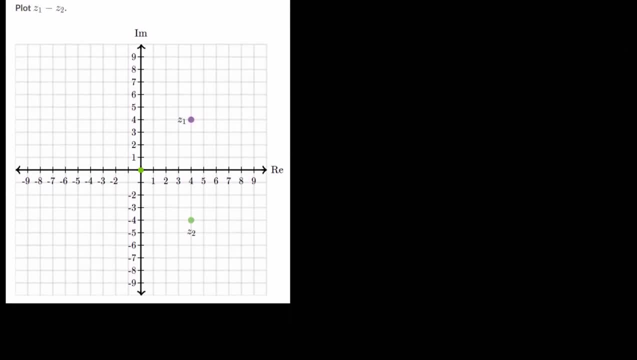 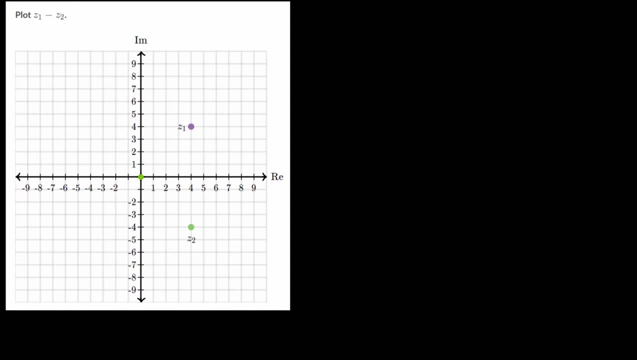 problem, And for this one we are subtracting z1 minus z2.. So let's start by writing both of these complex numbers in terms of their real and imaginary parts, And z1 looks to be at 4 plus 4i, while z2 looks to be at 4 for the real part. and 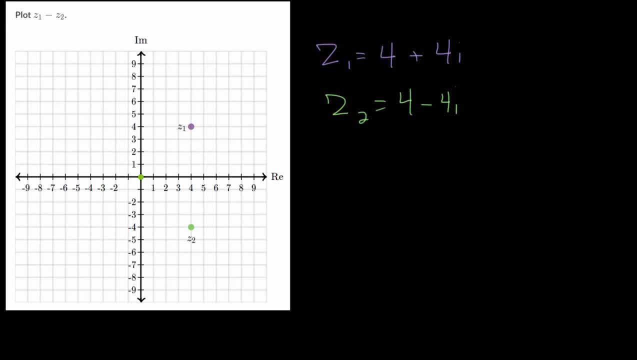 minus 4i for the imaginary part. And if we want to find their sum, then we take z1 and subtract z2, excuse me, we're finding their difference, not their sum, And we know z1, we can rewrite that. 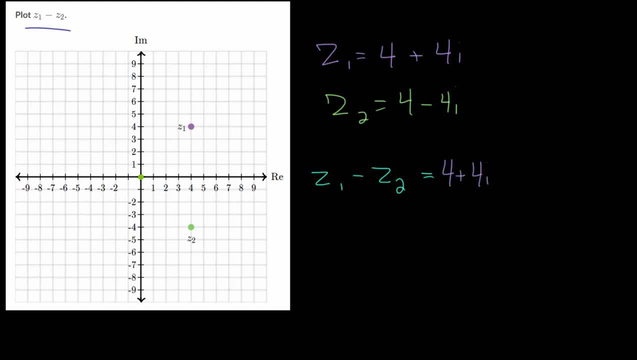 as 4 plus 4i, And we're going to subtract z2, which is 4 minus 4i, And I recommend writing this in parentheses, since we need to distribute this negative. We're subtracting the real part and we're subtracting 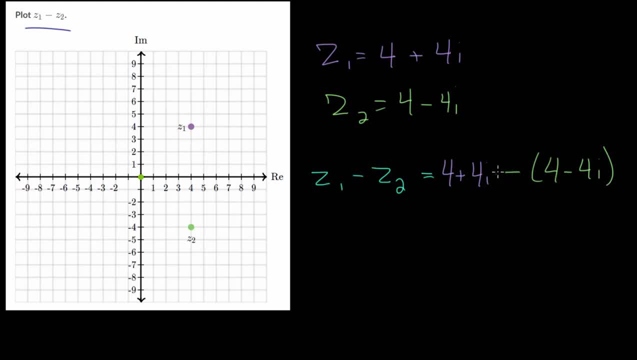 the imaginary part. Or, in other words, since we're subtracting a negative, we'll be adding the imaginary part And now just rewriting it without this negative. we will distribute it. We have 4 plus 4i minus 4.. 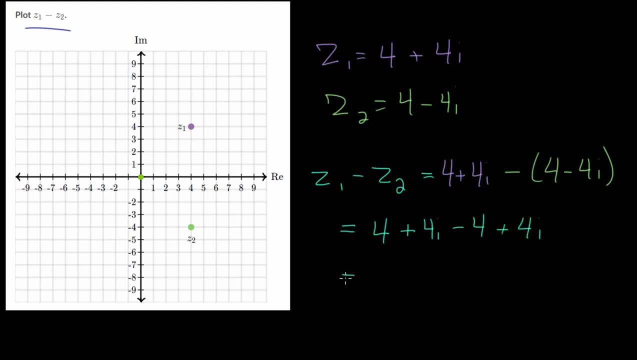 Plus 4i, since we are subtracting a negative. And lastly, combining the real parts and combining the imaginary parts: 4 minus 4 is 0 for the real part And 4i plus 4i is 8i for the imaginary part. 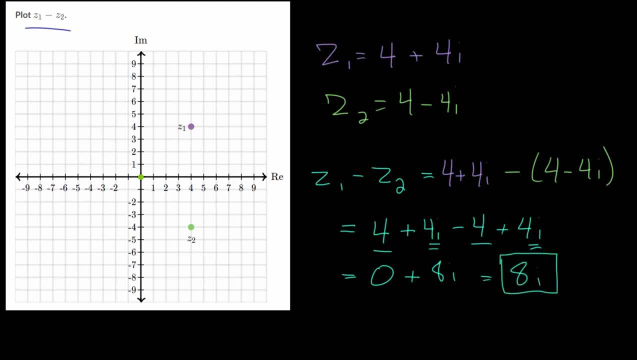 So this is a purely imaginary number And if we wanted to graph that, that would be right up here. But we can also approach this using vectors. We can check our work And the vector 2z1 will look like that And you can draw the arrow in if you want And the vector 2z2 looks. 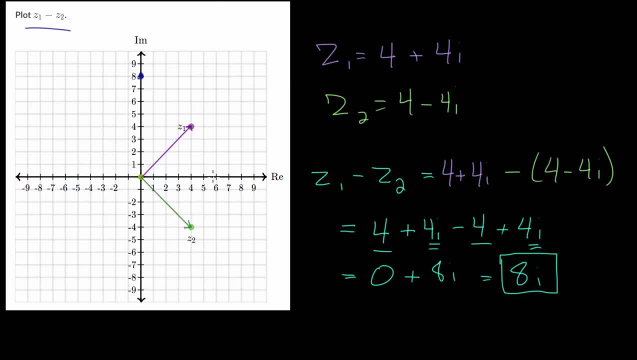 like this- Now with subtraction, remember, it's a little bit more complicated. Essentially, we want to find the opposite of z2 and then add that to z1.. And the opposite of z2 will be the vector that has the opposite real part and opposite imaginary part. Or you could think of it as: 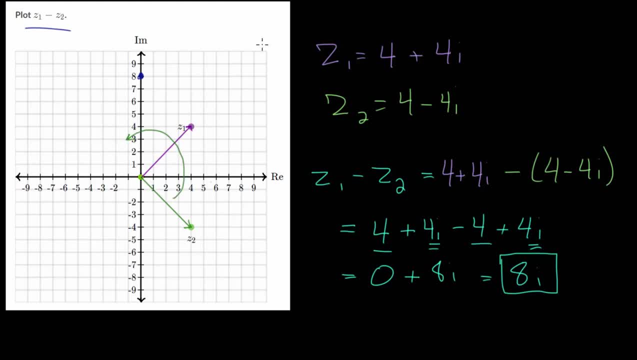 rotating this vector. So we will draw that vector 180 degrees and that opposite vector will continue along on a straight line. But we can find it by just finding the opposite real and imaginary parts. So it's the opposite: real part is negative 4, the opposite imaginary part is 4, which brings us right about there. 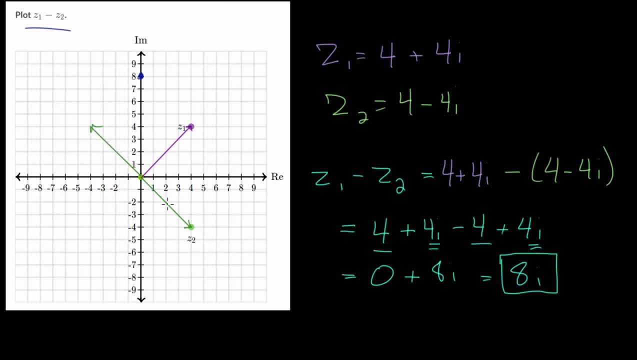 And notice it's not drawn perfectly, but you can roughly see that this is a straight line And let's label this. This is the opposite vector of Z 2, and now we want to add this vector to Z 1, so we're going to take this vector and slide it. 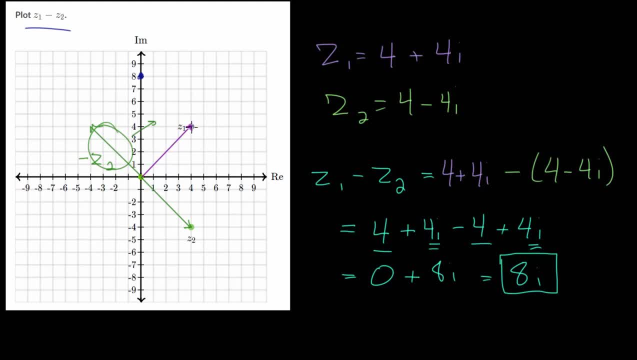 along Z 1 so that its starting point is at the ending point of Z 1 and starting at Z 1, we go left 4 and then up 4, and you can see our difference goes from the beginning of the original vector, Z 1, and to the end of the opposite of Z 2, or essentially where this